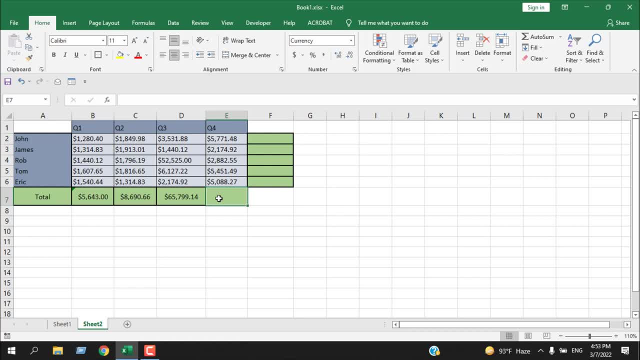 Now select the cell where you want the total. press alter and then equal to Now. this is the keyboard shortcut. Press enter for auto sum, and it will still work the same way. Press enter and it's done. Now if you want to find out the total for an entire row, you can use the exact same. 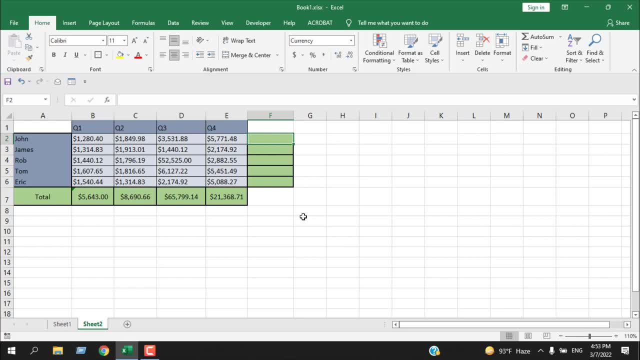 procedure I have used here, So I am going to simply show you the keyboard shortcut again. alter equal to. and it's done. Press enter Now. if I drag the formula, you can see it's working. So this is how you can automatically sum up an entire column or entire row in Microsoft. 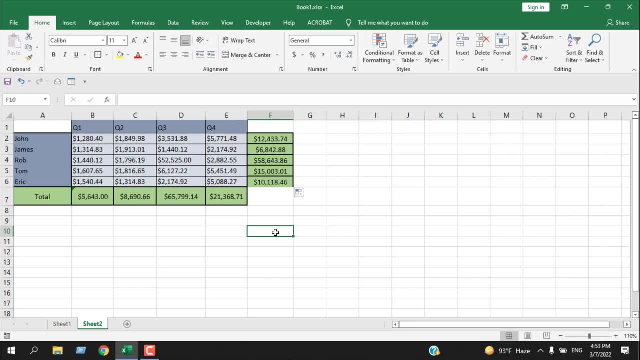 Excel. That's all I wanted to show you, Thank you. Thanks for watching. See you in the next tutorial. 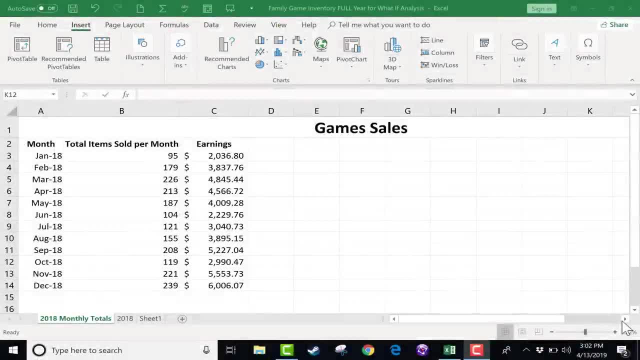 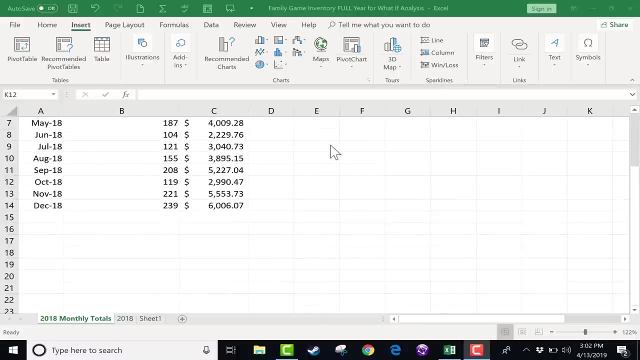 In this Excel tutorial, I'm going to show you some techniques and tools that we can use in Excel to identify trends, to look at how things are trending both in the recent past as well as looking toward the future. So let's get started. As you can see, I'm in a spreadsheet called Games. 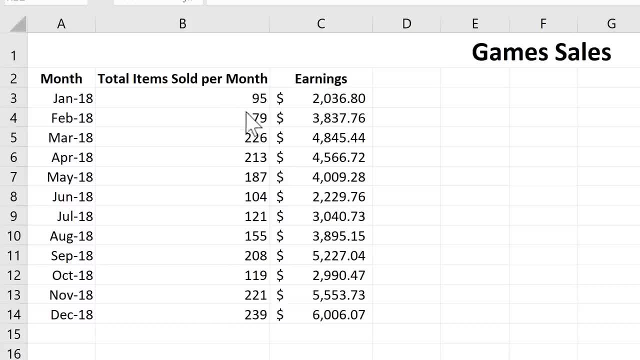 Sales and this spreadsheet tracks the total number of items sold each month for a small business that sells board games and card games. It also tracks the earnings that came from those sales and you can see each month is listed separately here. So the first thing I would 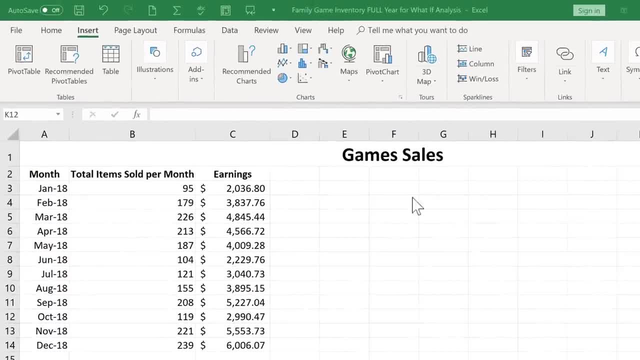 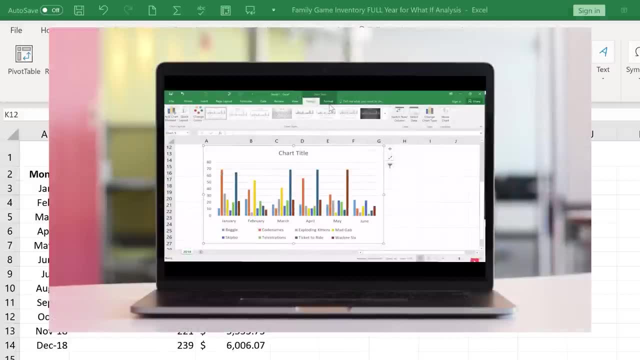 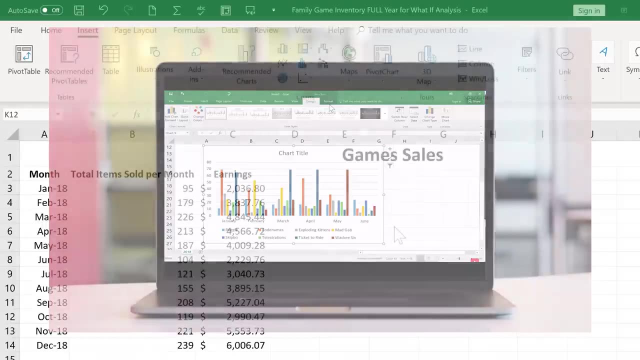 like to do is add a chart here at the right, and I'd like this chart to show the trend. How are the earnings trending for this company? In a previous video I showed some quick and simple techniques for adding charts to Excel, and if you haven't watched that video already, please do so. But in 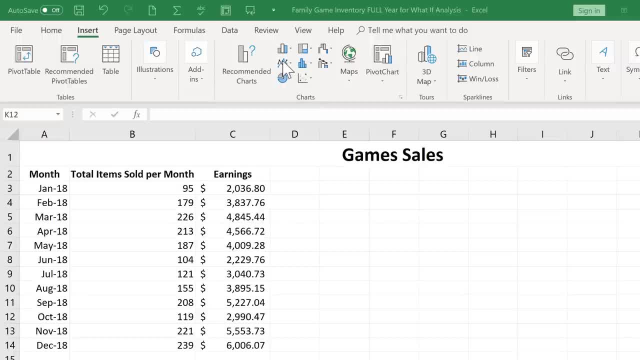 this tutorial, I'm going to show you how to add charts to Excel. I'm going to show you how to add charts to Excel. In this tutorial, I'm going to show you how to add charts to Excel and, if you, I want one specific kind of chart, this kind here, that's, a line chart or area chart, And the